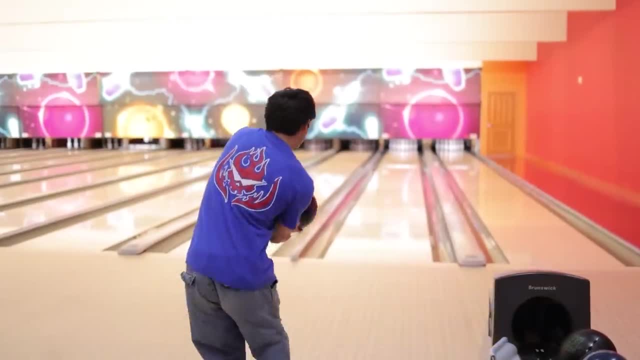 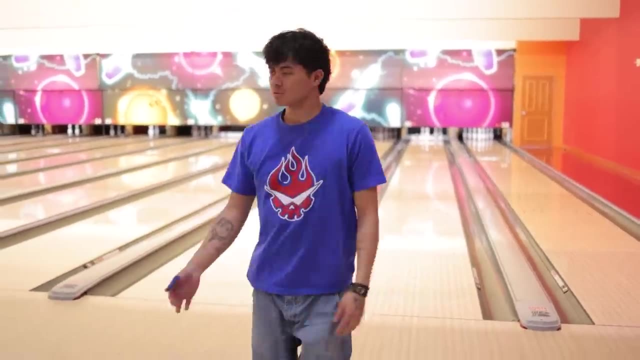 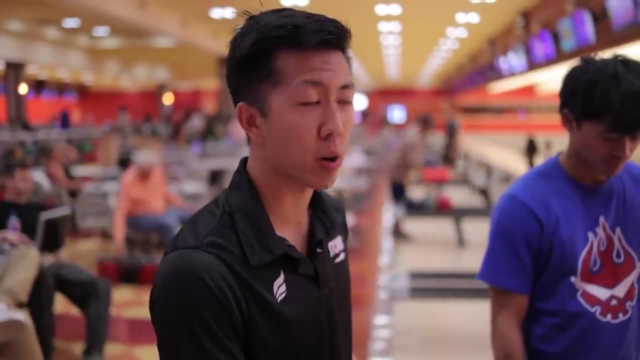 to target today with tip number one. Now, if you guys need a little bit of time to go back and watch the video again, go ahead and do that. Go into the comment section. let me know what you think he needs to work on his number one thing other than hit the one in the. 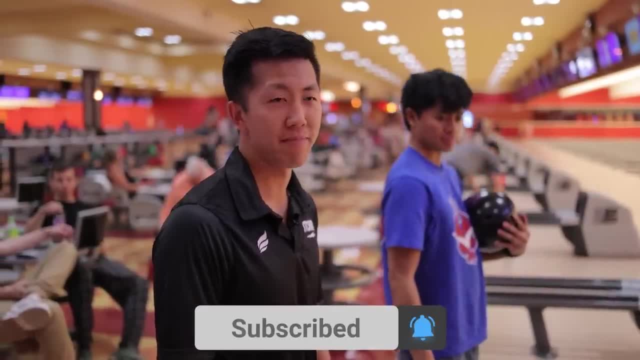 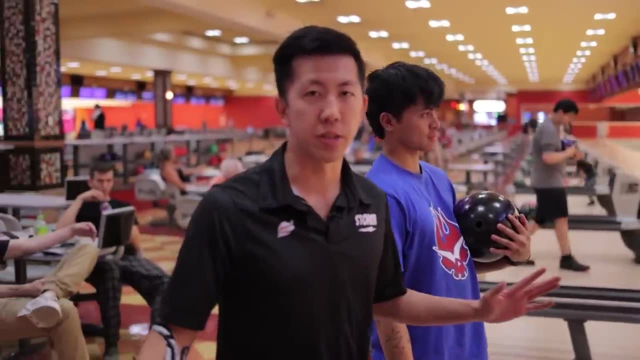 front: Alright, did you get it? If you did, awesome. If you didn't, that's okay. We're here to learn. This is gonna be tip number one. So what Kyle does in his approach is very common amongst a lot of amateurs that I've worked with in the past, So I'm 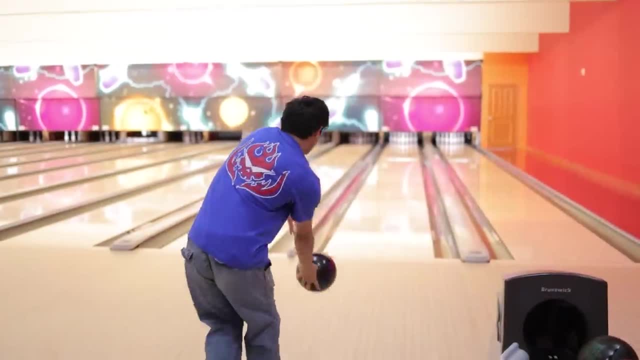 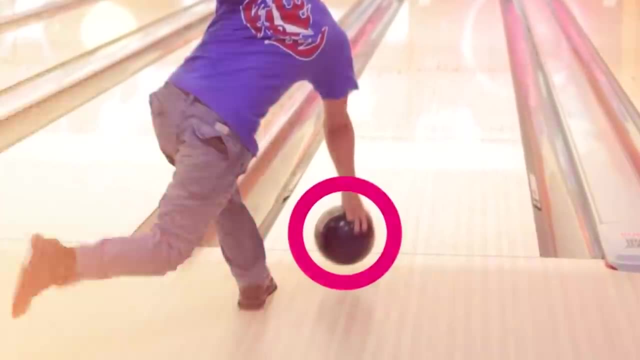 assuming that this might apply to you as well. When he gets into his wing, the ball gets way too far behind his head And it doesn't allow him to get his hand behind the bowling ball like a lot of the PBA Tour pros. What we're gonna try to adjust today is get that ball. 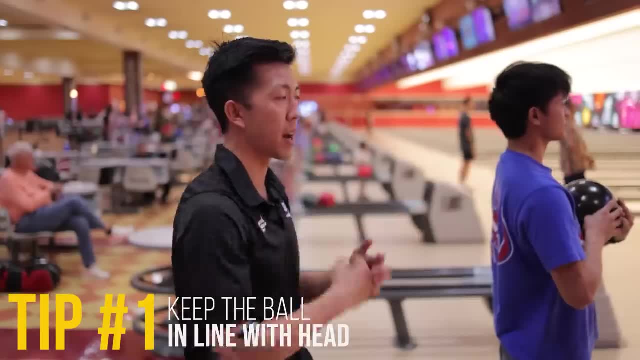 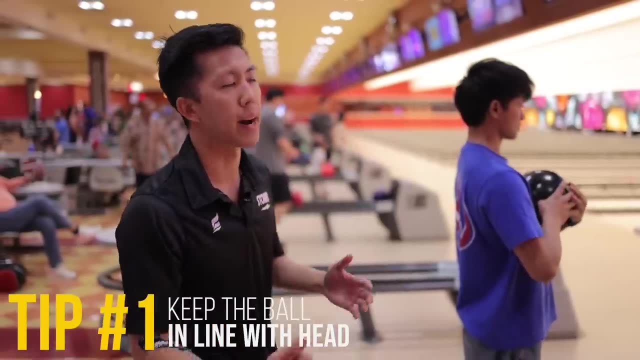 position a little further behind his head instead of too far inside, Because when it gets too far inside, the only way to go is the out. It comes around the body. We don't want that to come around the body, because when you get your hand, 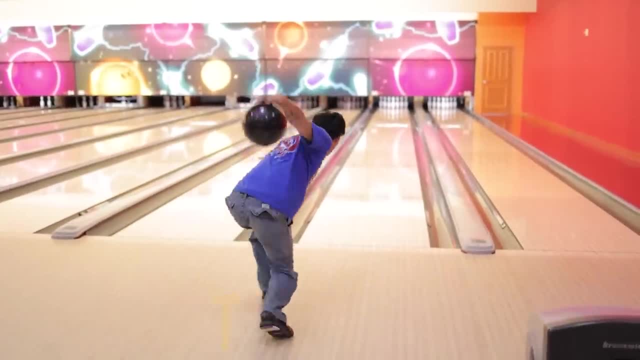 on the outside, on top of the ball. it's a very weak position and it's hard to create power. So if you want to hook it like the pros, you got to get your swing a little bit straighter so you can work the inside of the bowling ball. That's. 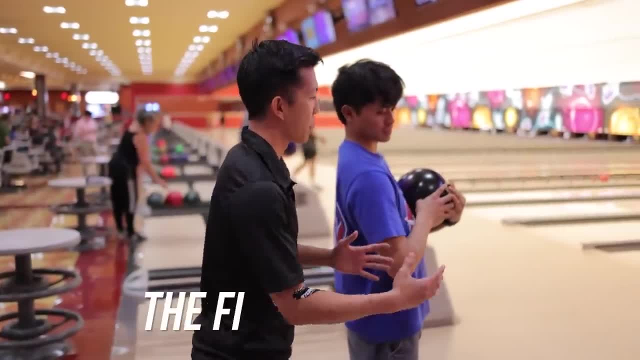 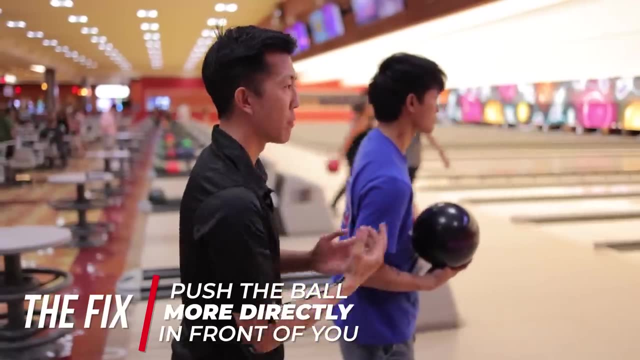 what we're gonna try to do here Now. what I want Kyle to do is to push a little more in front of him. So when you push to the right, that allows the swing to follow that direct path. So if it goes to the right, the swing's gonna end up behind you. So if we get that swing a 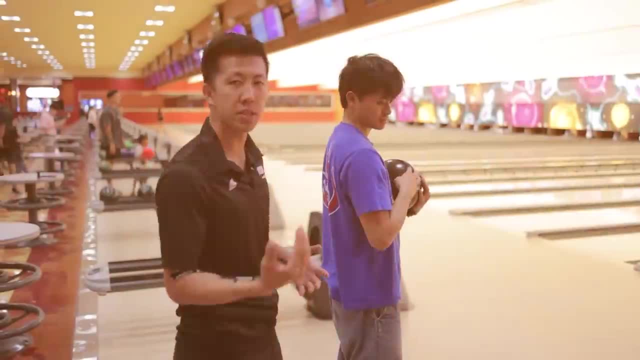 little more in front of him. hopefully it's gonna line up with his head a little bit better. The goal is to get his push away straight. So what I'm gonna have Kyle do is visualize pushing to the left. Now what you might notice is the. 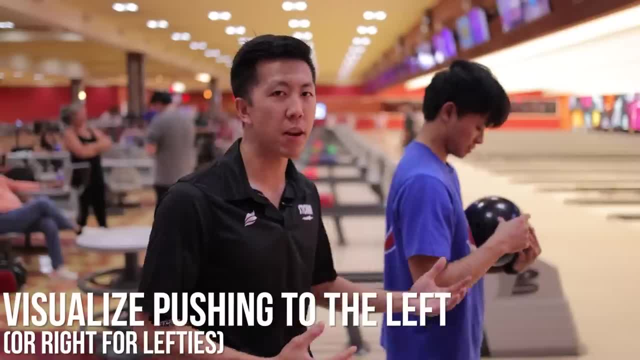 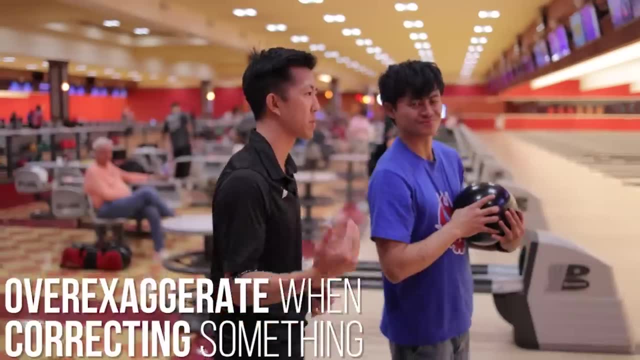 swing. if he accomplishes pushing it to the left, it might look straight. It's never gonna be exactly what you envisioned it to be, So you always want to try to over-exaggerate it as much as possible. So we're gonna have Kyle try to push to the left and we'll see where his swing. 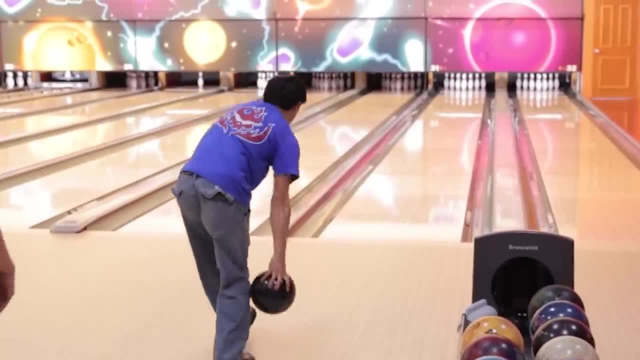 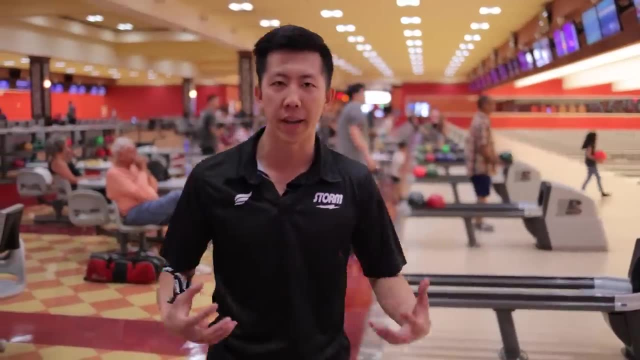 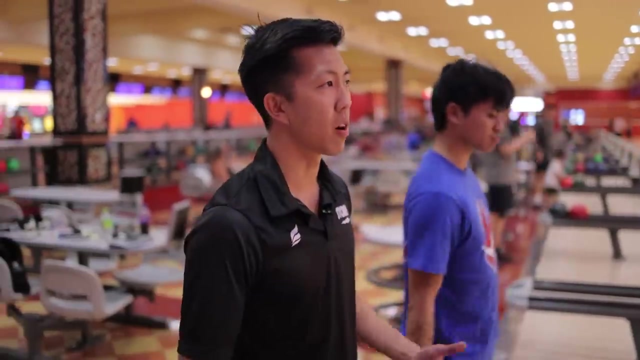 ends up at the top. Now, Kyle probably felt a little bit of an adjustment. His body's freaking out, going hey, what's going on? And that's what you always want. You want to trick your body, because your body is always gonna do what it's used to doing. So I 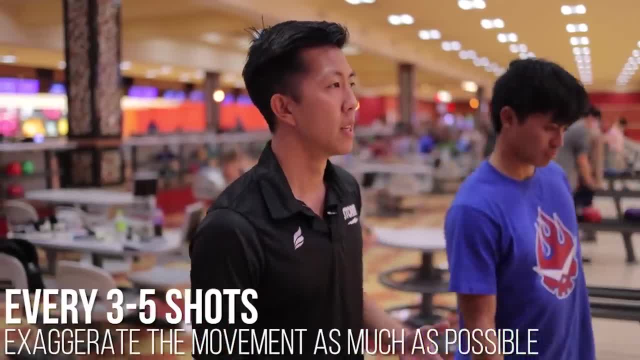 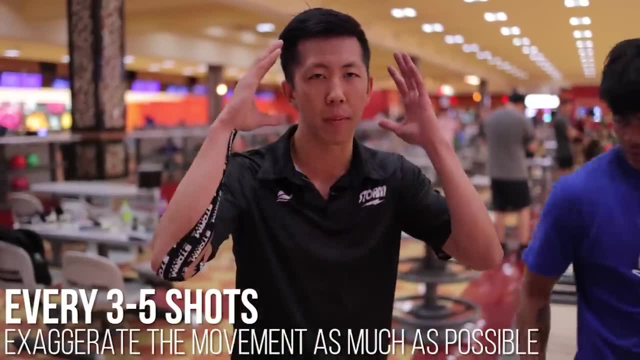 would say every handful of shots, maybe three, four, five shots. you want to overdo it. Remind yourself, hey, I'm working on this. let's do this Because if you just keep throwing shots and you just keep thinking about the same thing, eventually. 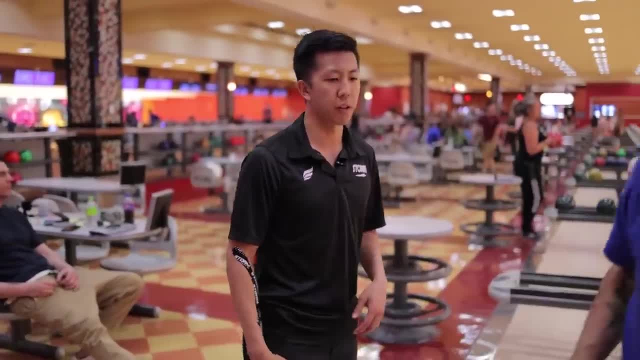 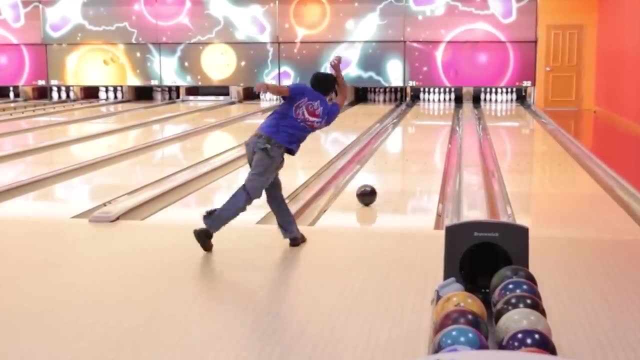 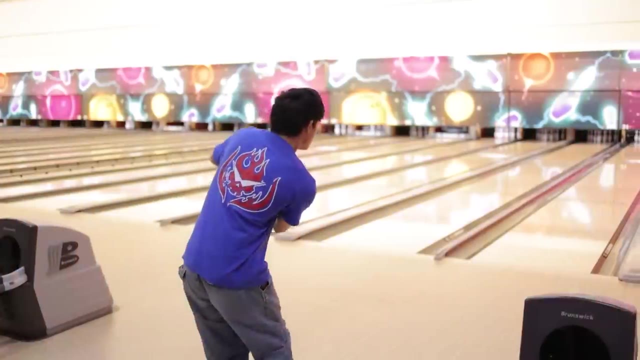 your body's gonna catch up to you. All right, Kyle. now let's really over-exaggerate this. I want you to feel like you're pushing away to the left, and then we'll see where your swing ends up. Now, sometimes we could push things a little too far. You see how far left he. 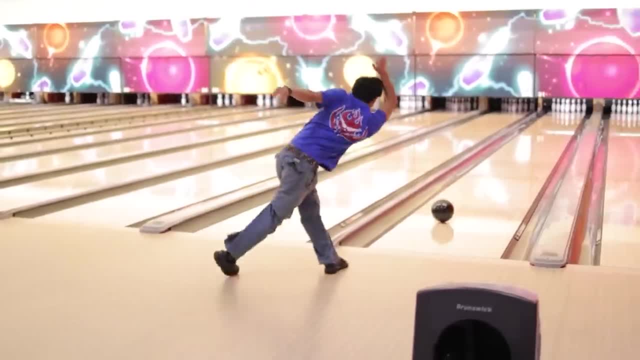 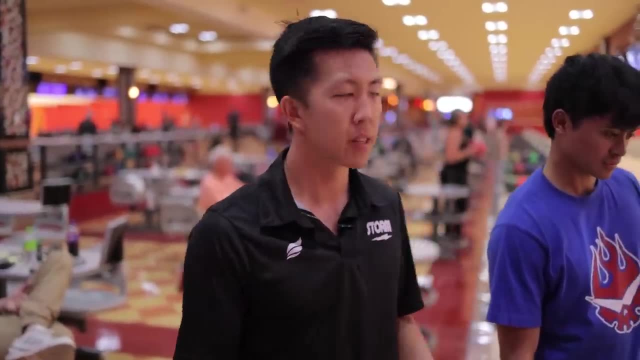 actually got it going. Now he created a really big figure-eight swing and that's kind of getting away from what we want to accomplish. So depending on who you are and how fast you're able to fix things, you know I've worked with people that are very mendable. like Kyle can just do things on command. 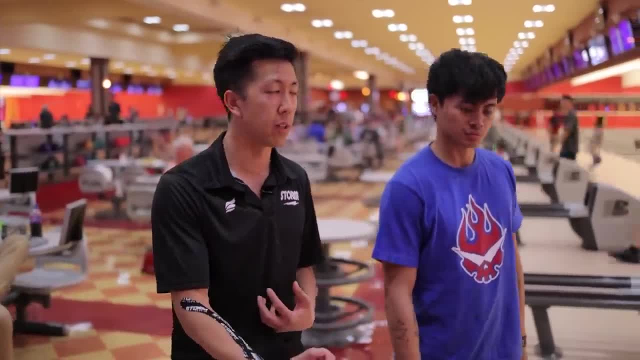 and other people have a really hard time getting their bodies to do what they want it to do, Depending on who you are. you just got to figure out how far you need to go. If you're overdoing it, just dial it back, And if you can't, if you're 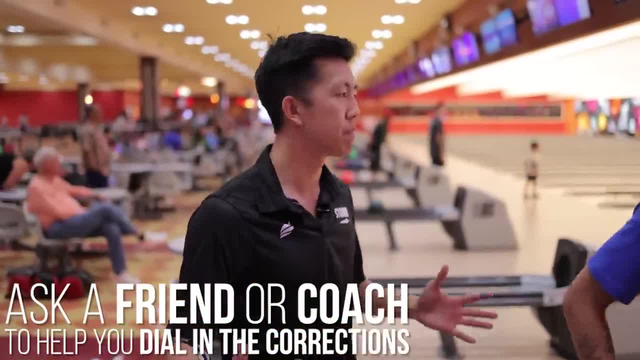 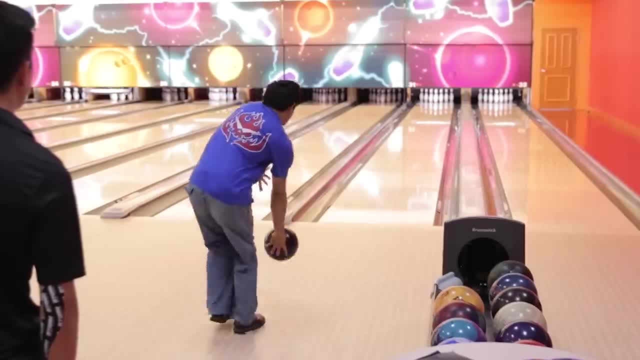 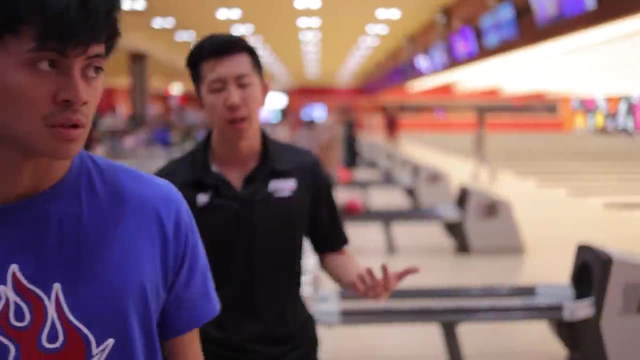 having a hard time getting that feeling. maybe have somebody else with you to push you in that direction. All right, let's dial it back a little bit, Stay nice and loose with the swing and keep it nice and straight. And again, it's not going to be an overnight process, You know. if you don't, 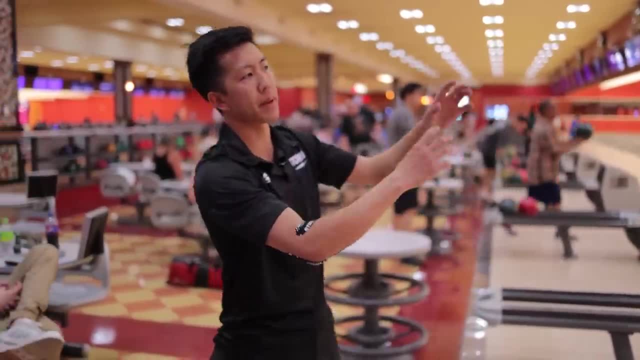 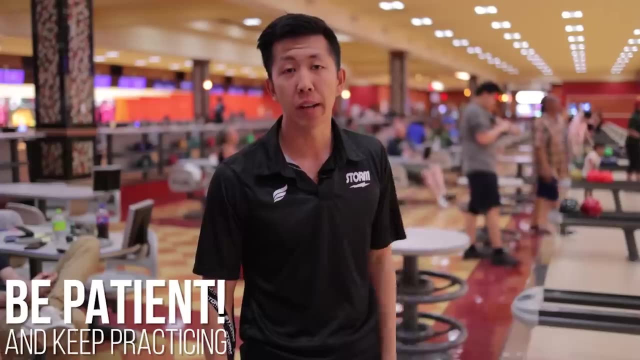 see Kyle making that immediate switch. you know that change where the ball may be a whole ball inside of his head. it's not going to directly line up on the very first day. It's something that we're going to work on continuously. It'll get there one day as long. 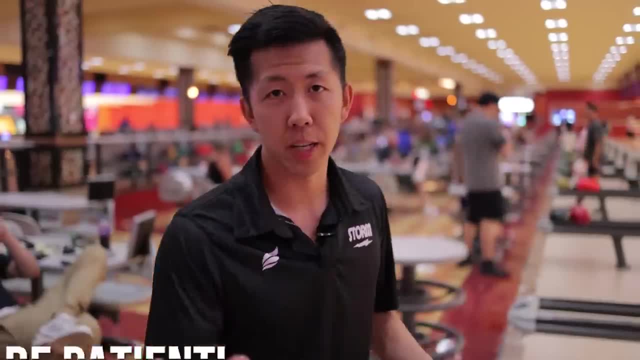 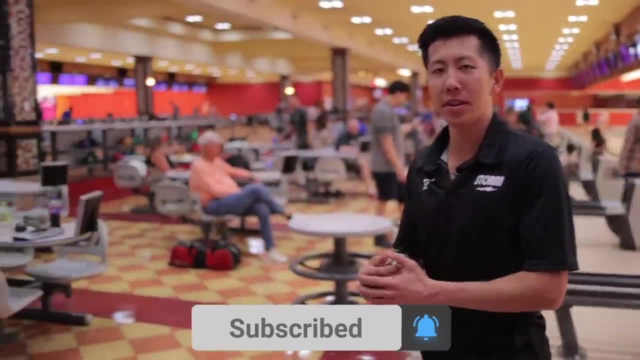 as he works hard And that's the main thing: just keep working hard. I want you guys to make sure to stay around for this final tip, because it's probably the most important one out of all of them. So for tip number two, we have Chris. You may have seen him before. He's been doing. 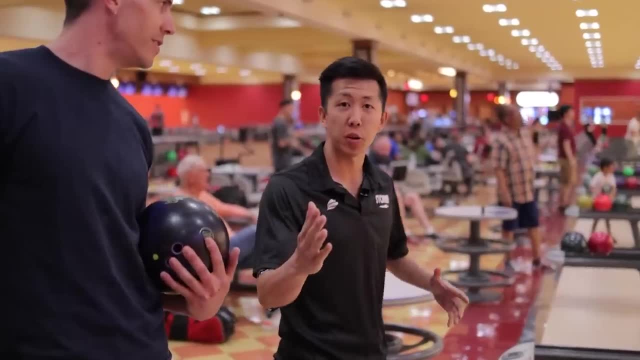 a great job. He made an appearance in ProVAM and he's been wanting a lesson, So we're going to do the same thing as earlier. I want you to guess what we're going to work on with Chris today. We're going to have him throw a shot and let me know in the comment section. 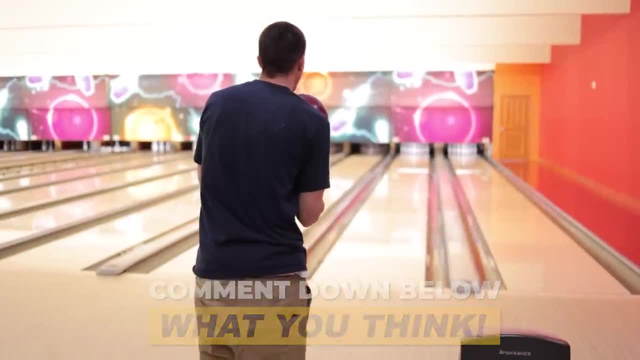 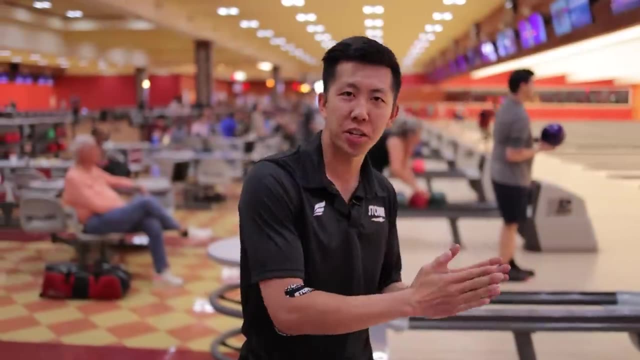 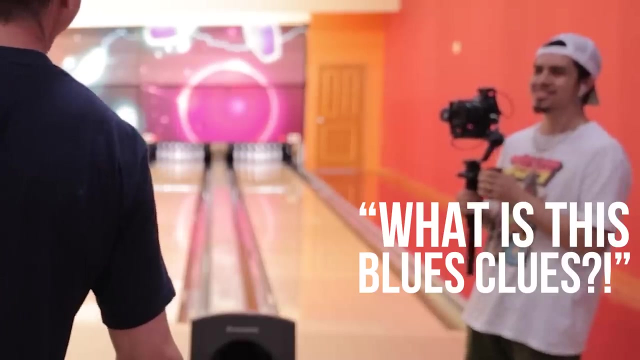 what you think that we're going to work on with Chris. Rewind the clip. watch it over again. Let me know in the comment section what you think. Did you get it? No, Yeah, If not, that's how you prefaced it. 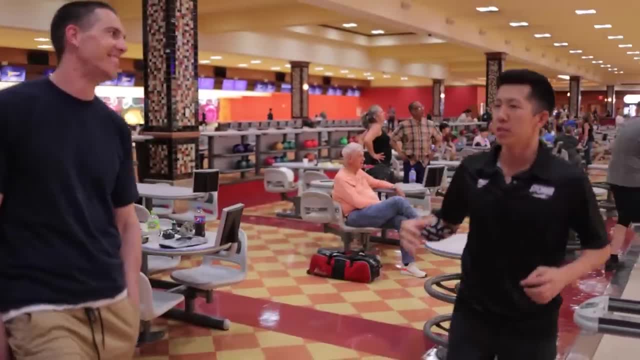 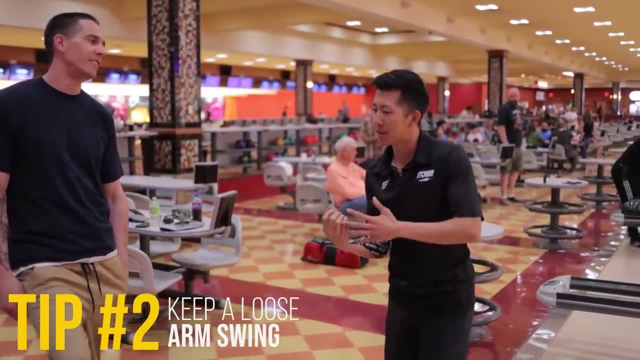 All right, Chris. So what I've noticed is you're a little inconsistent. Absolutely, I want you to loosen up that arm swing So we're going to get to the apex or the peak of the push. Once you get to here, I just want you to feel nothing. I want you to loosen. 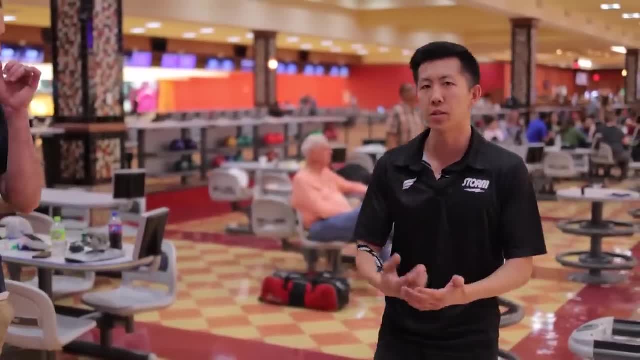 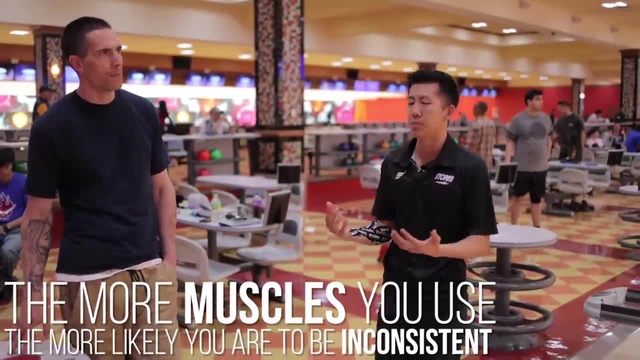 up that swing. That's going to allow you to be more consistent, because loose muscles are fast muscles. The only way your swing is going to get offline is if you introduce some external forces. Yeah, Yeah, So it's basically muscling the swing. This is also very common in most 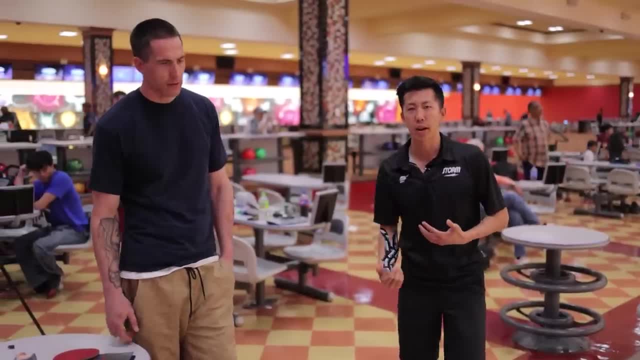 lessons I've given. So that's one of the main things that I try to really enforce is just having a loose swing, So give it a shot Again once you get to that end of the push. just let it drop Consistency. 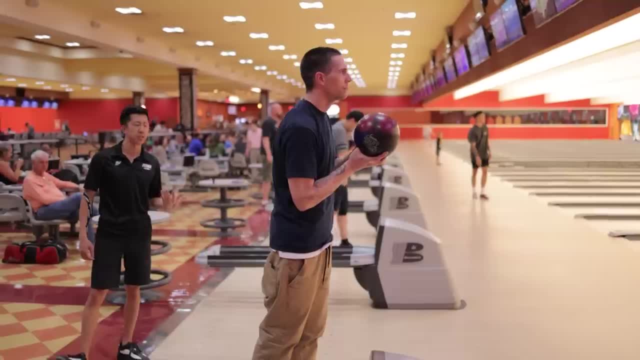 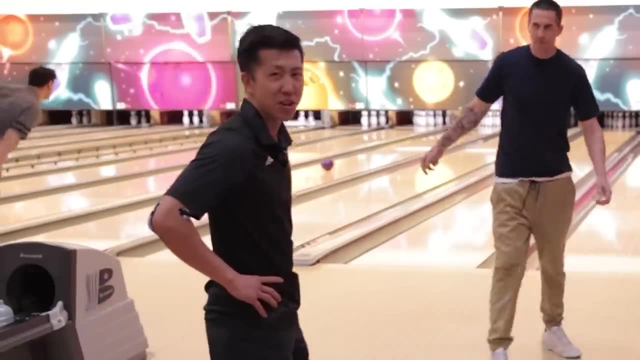 is one of the main concerns when it comes to lessons and trying to improve, And it's a really good way to do it. Look at that: That's the most ball motion you've seen all day. Yeah, it actually shaped up really good. Chris actually struggles with getting his. 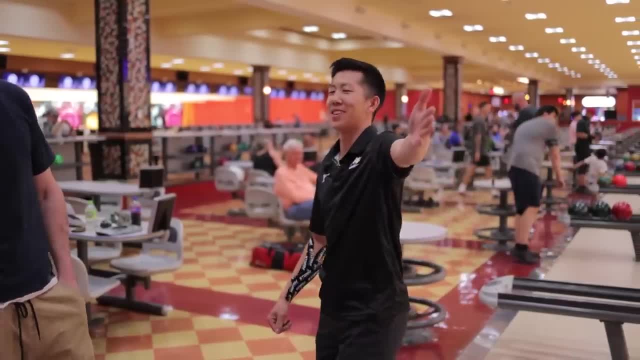 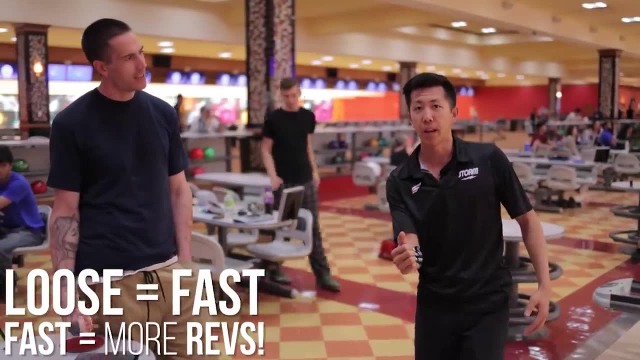 ball to hook And Jesse always keeps pounding it into him. because Jesse sees it more often than I do. He's like: throw it slower, man, Throw it slower. What Chris may not know is that when you get looser, your hand moves through the ball faster, And when your hand moves through 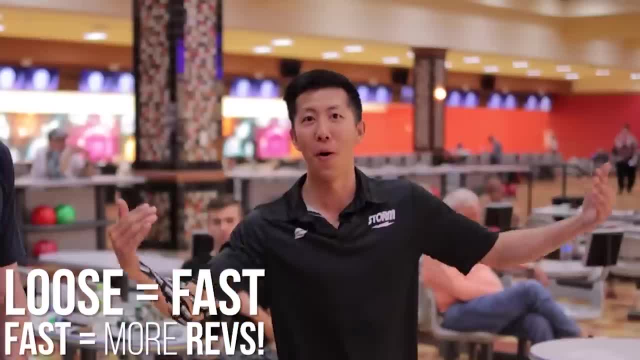 the ball faster, you create more reverie. And what does more reverie give us? More hook. All right, Chris, let's try again Now on this one. I want you to give me a scale of one to ten. how loose you feel on this one? 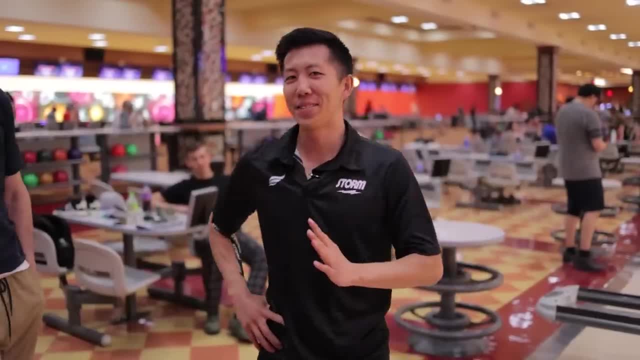 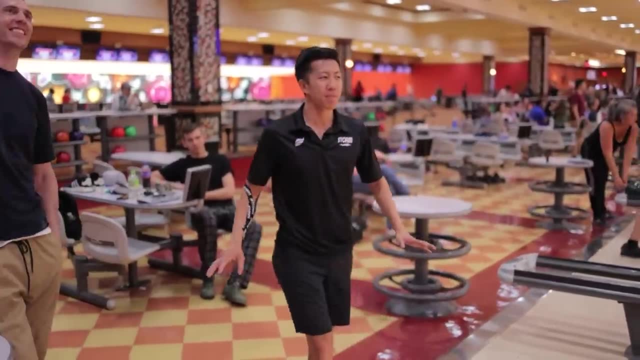 About an eight? About an eight? Yeah, All right. From earlier he was definitely like a one Pressure: Let's maul the holes, Let's just ugh. So he gave us an eight. I want you to. 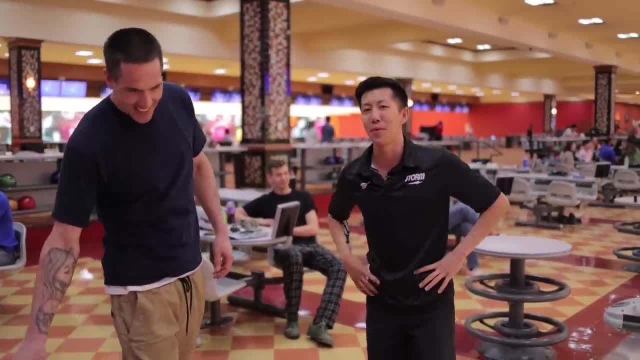 feel like a 16. 16. I always double it. You know, normally people are pretty realistic with themselves. They're like, yeah, it was like a five, But he gave himself an eight, So make it feel like a. 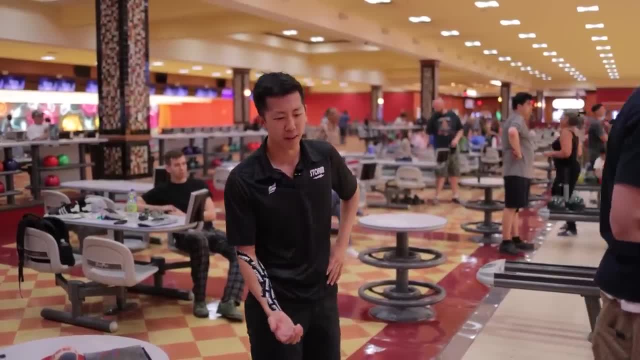 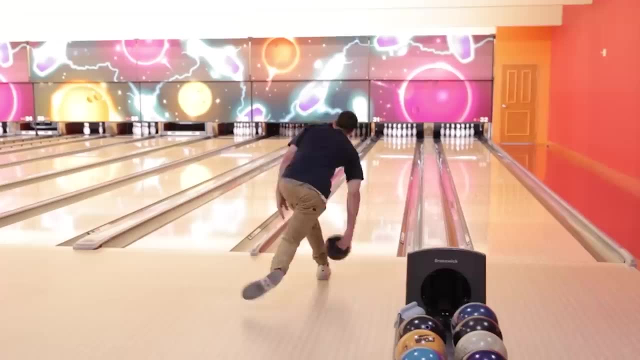 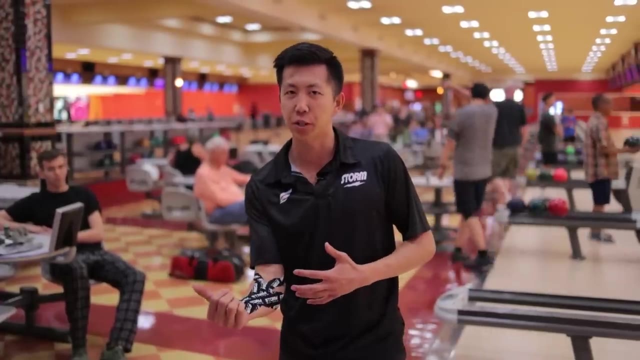 16. A 16 out of 10. Almost feel like you're going to drop the ball. I don't want you to drop it, But if you do, that might be a fit issue. All right, He didn't get quite good out of that one, As good as the first two, But the first two did shape. 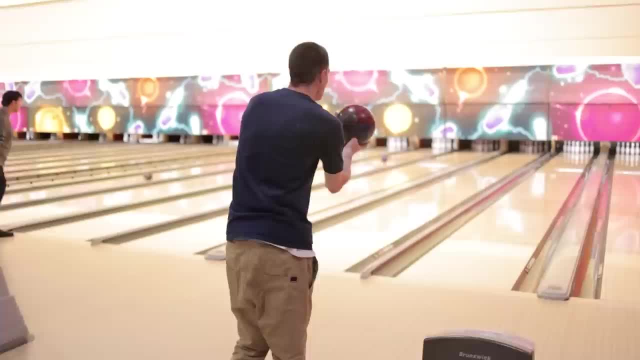 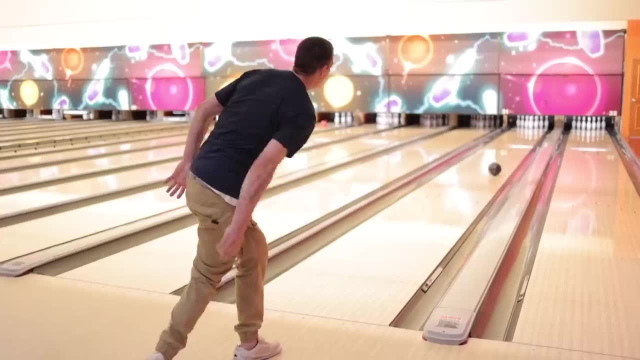 really well And all he did was loosen up his swing. So if you're trying to hook it more, maybe that's one thing that you do. Just loosen up your swing Helps with consistency. again, Repeating shots is the number one thing in this game. We're going to have Chris throw some more. 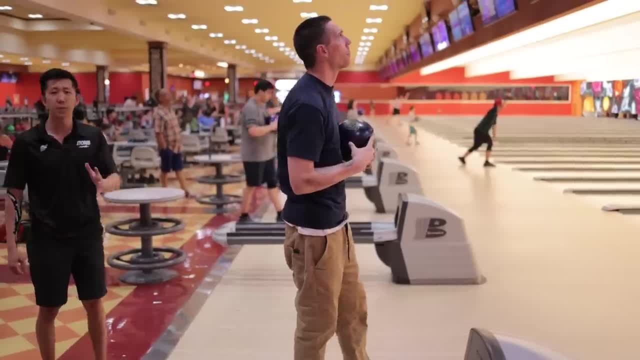 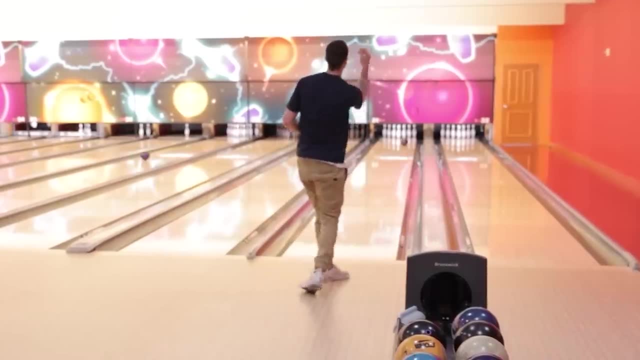 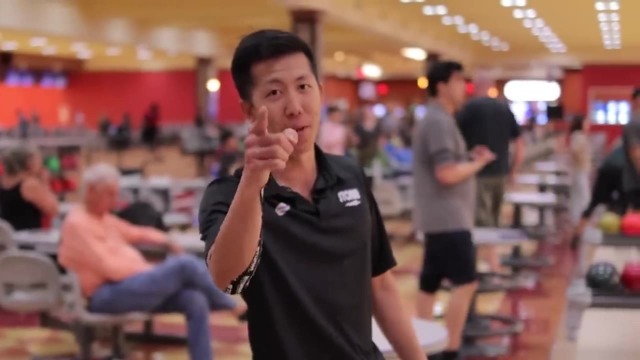 shots and just try to get as loose as humanly possible. Every shot's been fairly on line so far as well, And that's what we're looking for. Are we good to go? He's thrown three really good, Good ones. they've all struck. Oh wait, There's one more tip, The most important one. So we've 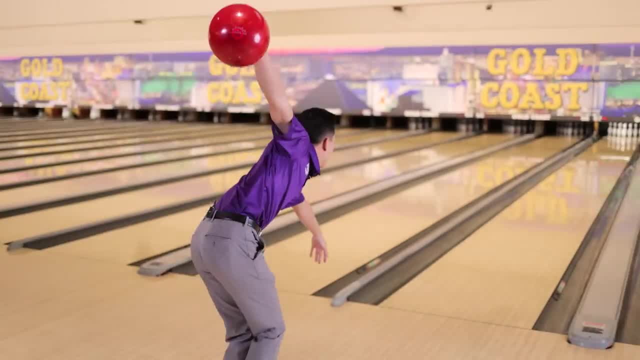 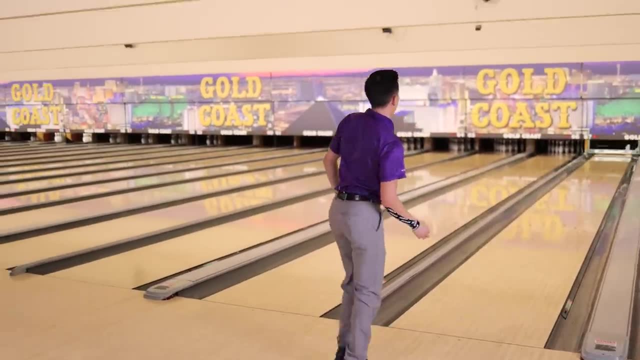 given you two very, very valuable tips so far. Swing direction is really important, Being loose as well. Those are the two key components to being consistent. Looseness, consistency: straight loose, straight loose. But we got one more for you: We're going to bring Aiden in here And again. 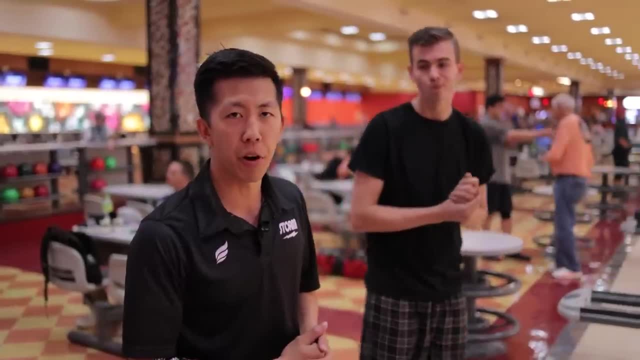 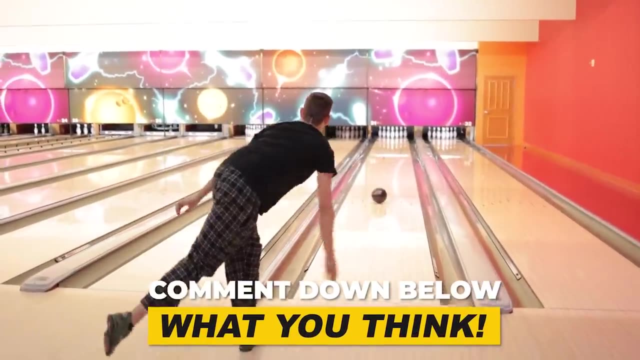 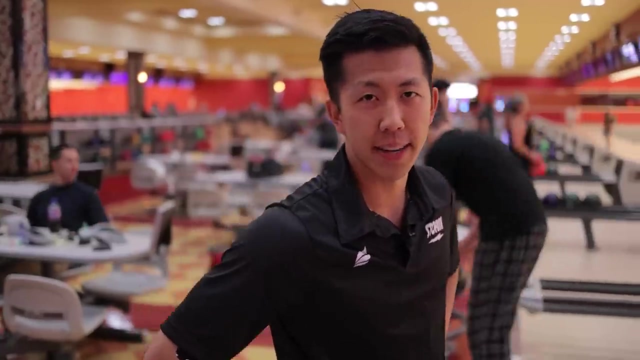 I want you to guess what you think we're going to work on with Aiden, And this is going to be our third and most important tip of the day. How good are you? Do you think you know what we're going to work on today? Again, rewind the video. 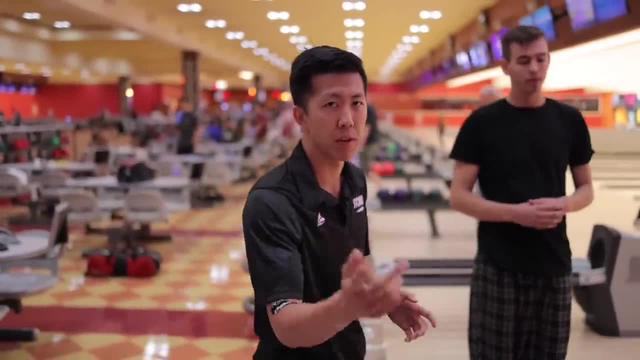 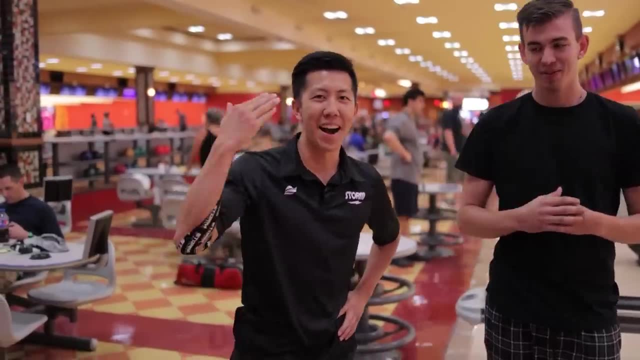 watch the shot again. Let us know in the comment section below. We'll give you a minute. Do you think you know what you're working on today? He's got no clue. You guys have no clue. I have the only clue: It starts with a, B and it's not bad. We are working on balance. Balance is one of the 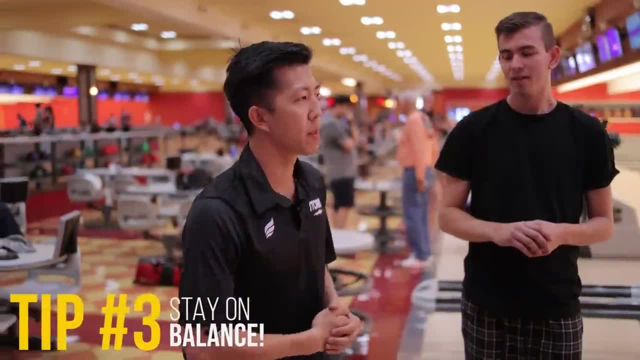 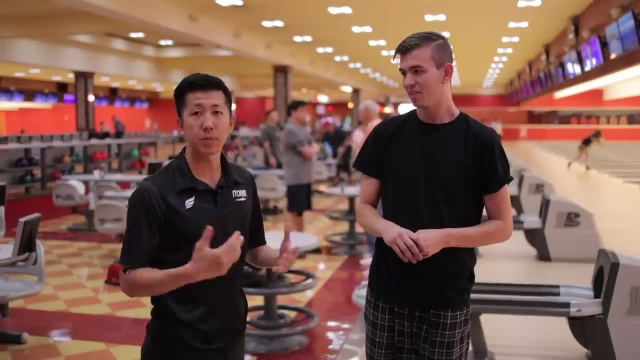 most important things in repeating shots. You add all the tips together, you're going to have a really good chance to shoot some really high scores. Nice statue: finish at the line, like Randy Peterson likes to say: Super corny. Sometimes it's just a conscious effort to just post your shot at the line, Other times it's you know. 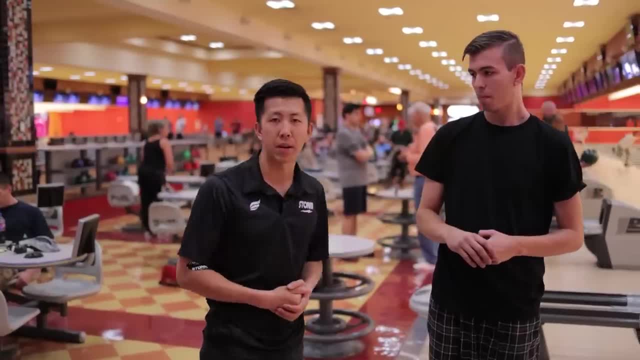 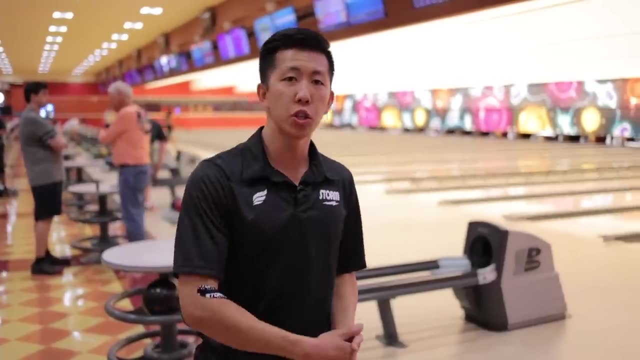 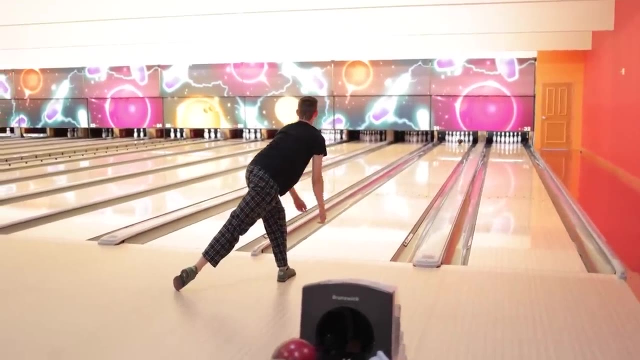 things throughout the approach that lead up to lack of balance at the line. So let's throw a shot, see what we can do. Throw it however you want. Try to post your shot the best you can. Now, tips one and two actually help a lot with tip number three, Really good Sometimes. 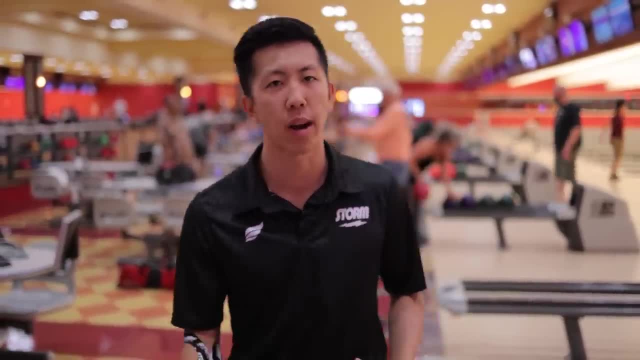 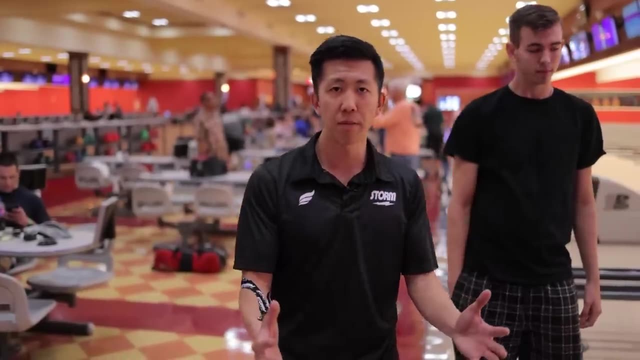 it really is just making a conscious effort. Sometimes we get so caught up in trying to hit it harder, trying to throw it down the lane as hard as we can, that we're not even thinking about the foundation If we don't have a strong foundation. 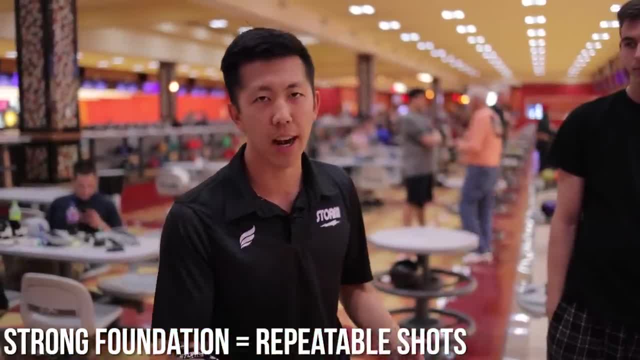 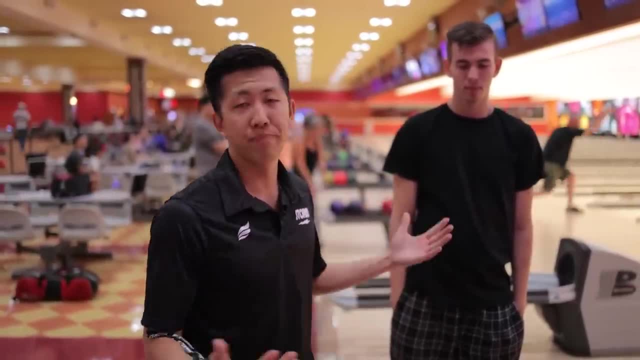 at the line. there's no way we can repeat shots, shot after shot after shot. So if you have a straight swing, a loose swing and good balance, those are all keys to success in bowling. If you look at almost every single professional athlete, every Hall of Famer, they've got straight swings. 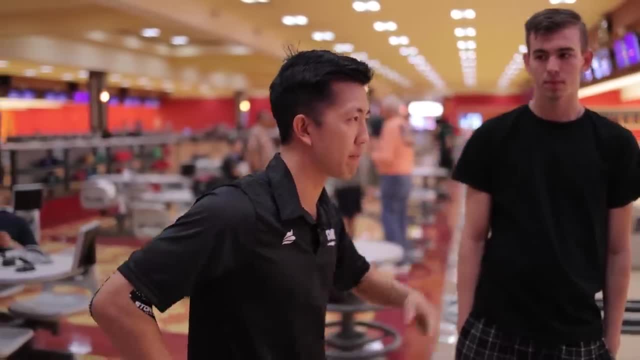 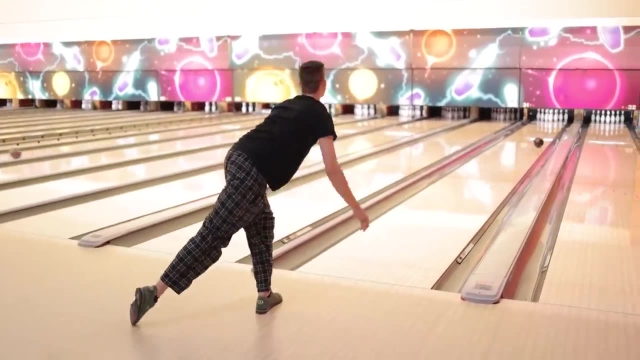 they have great balance and this is what we're trying to achieve with Aiden here Now. Aiden's actually been working on trying to hit the ball a little bit harder, so that can contribute to his lack of balance at the line. But so far so good. You know when you get to. 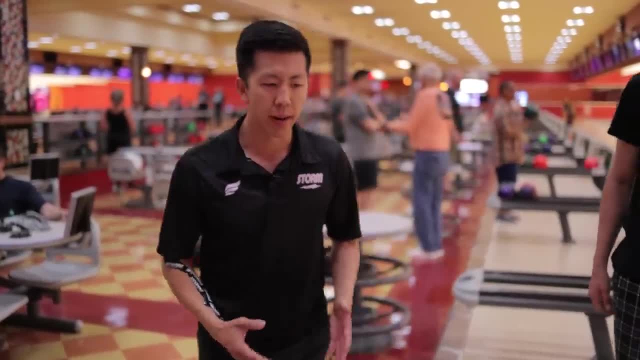 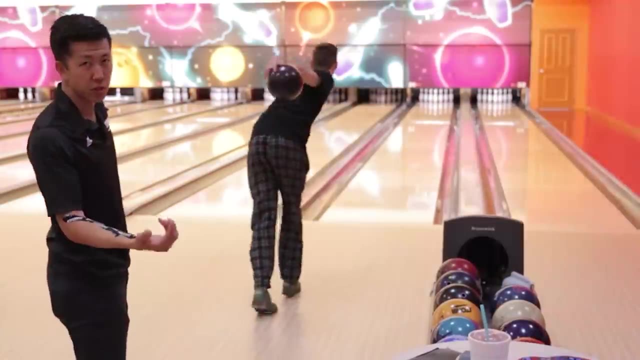 the line, things that really go into having good balance. you don't have a good knee bend. You want everything moving forward. You don't want to have too many pieces moving left or right. You don't want to get too twisted at the line. Aiden's doing a really good job of staying nice and forward with 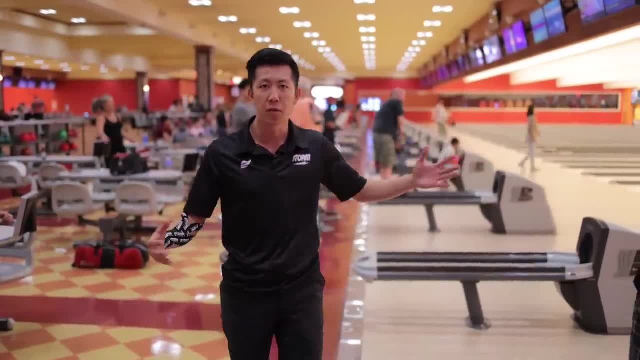 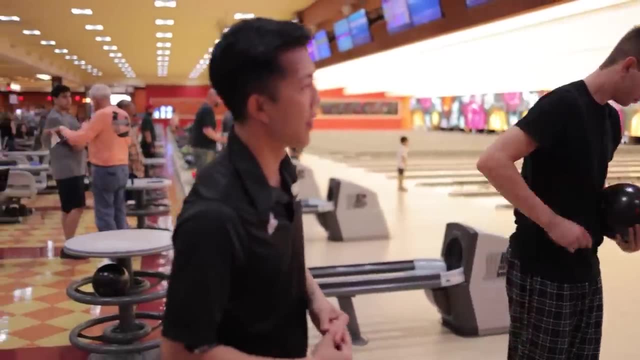 the lane, because the lane's actually a lot more narrow than it seems. So if you get pieces moving right, you don't want those lateral movements, because that's going to lead to inconsistencies, And that's not what Aiden wants, That's not what Chris wants, That's not what Kyle wants, That's. 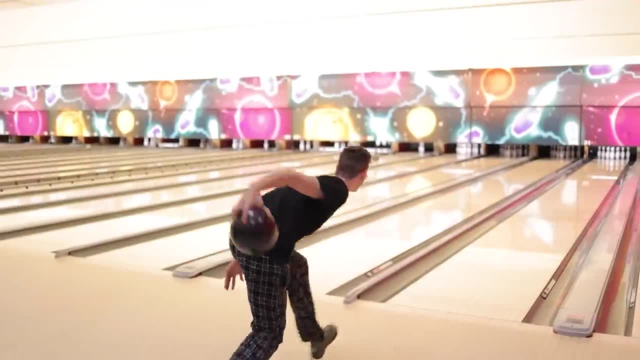 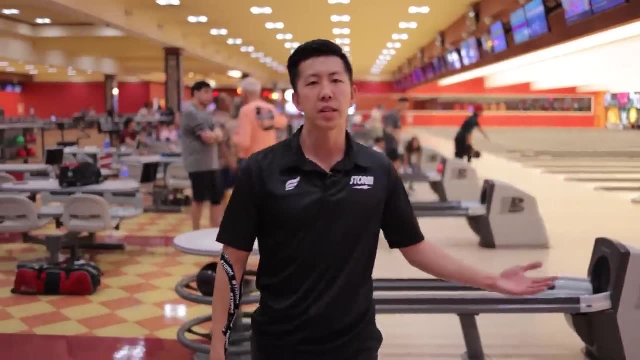 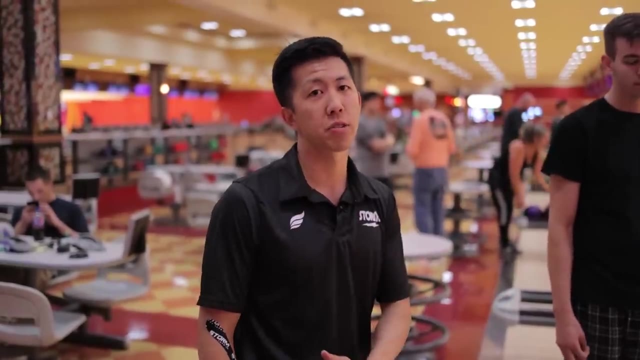 not what Darren wants, And Darren wants you to be great. It's great stuff. You know it's not always going to translate to the best results. Just because you post a shot doesn't mean that you're going to strike every time. But I guarantee you it's going to increase your chances of striking. 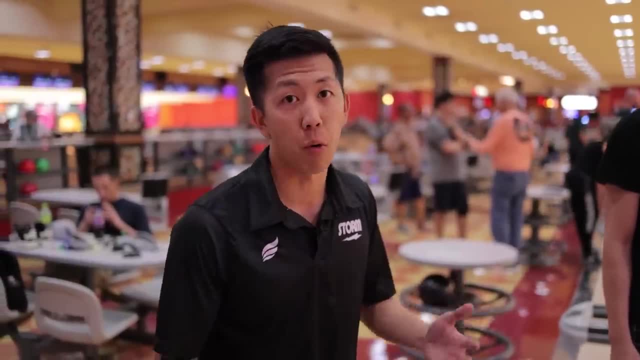 more often if you post your shot, rather than falling off Every so often all the time. All right, Well, that's going to do it for our three tips. Don't forget it. Tip number one: you want to have a straight swing, as straight as possible. Keep. 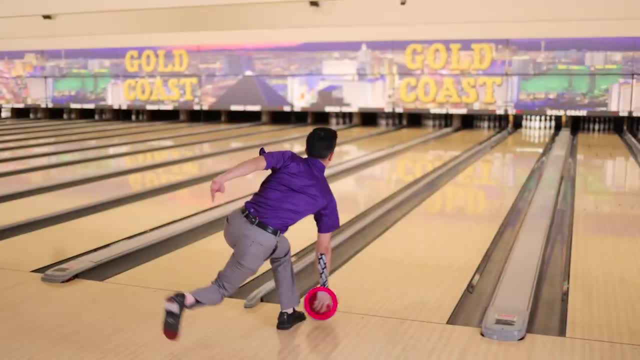 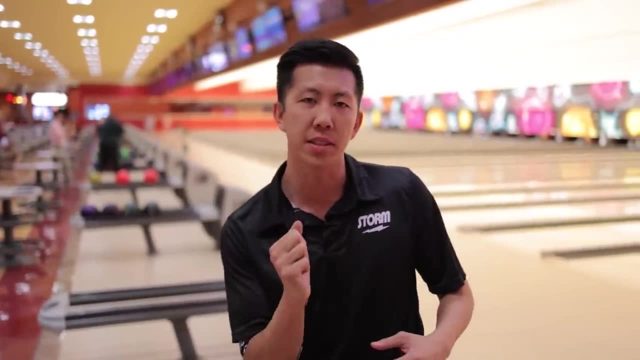 that ball nice and in line with your head. Tip number two: you want to be nice and loose because you can repeat more shots. if you're loose, If you're squeezing the heck out of the ball, it's going to be really hard to repeat that and get out of the ball consistently. And the most important, 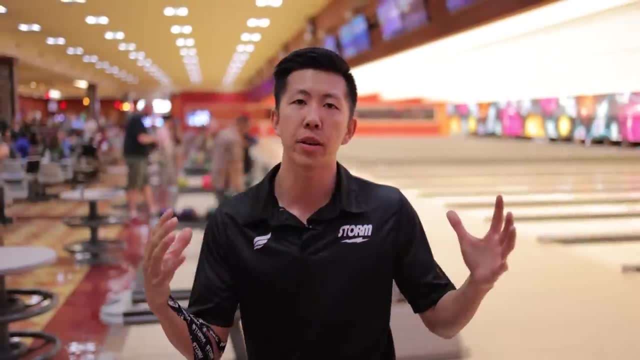 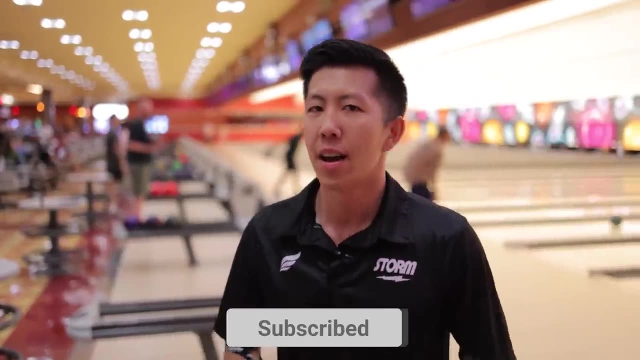 tip. tip number three is balance. You combine all three of those things, you're going to be very successful. I promise you keep working hard out there, guys. Thanks for watching. Hit that like button, like the video, because it helps the algorithm, and let us know if you want to. see more educational content. Thanks for watching.